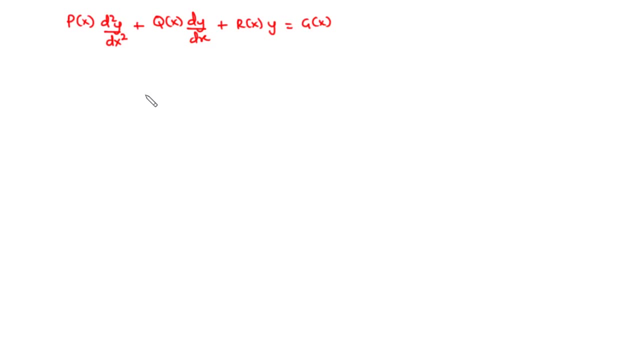 is said to be a second order differential equation. Now, a second order simply because the highest order of the differential equation is 2, and then linear, because the functions p, k, r and then g are all functions of x. Now, if the right hand side of this differential equation is equal to 0, then we say that we have a second order: linear, homogeneous differential equation. 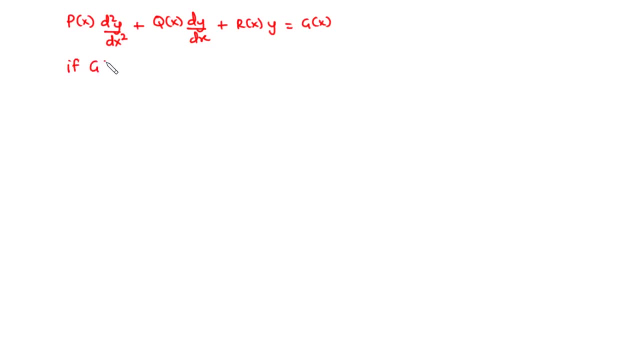 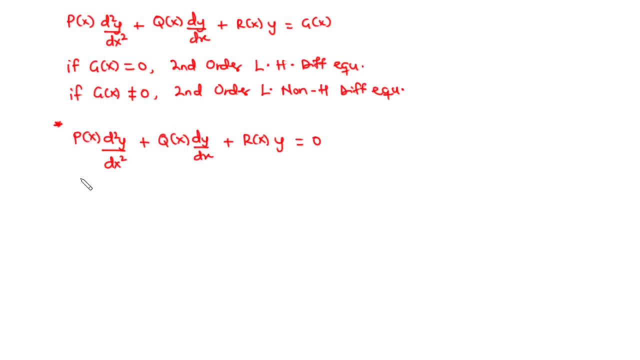 And how to obtain the general or the particular solution of such differential equations In prime notation. that is, we have: p of x times y, prime prime plus q of x times y, prime plus r of x times y equals 0. Now, considering that p, q and then r are all constant functions, or better still, they are constants. 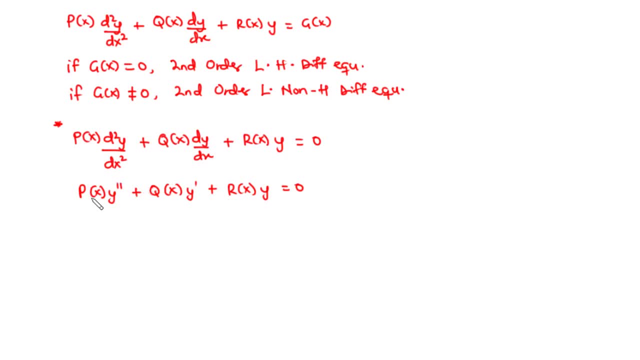 then we can represent the differential equation by replacing p of x with a, q of x with b and then r of x with c. Mind you, a, b, c are all constants. So we are going to have a times y prime, prime plus b, times y prime plus c, times y equals 0.. 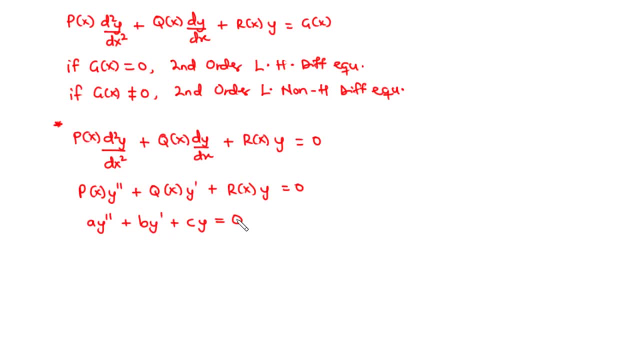 Now let's consider a trial solution. Let's assume that we are going to assume that the function y equals e to the power m times x is a solution to the differential equation. So it's a solution to the above differential equation. Now, if we make this assumption, then what this primarily means. 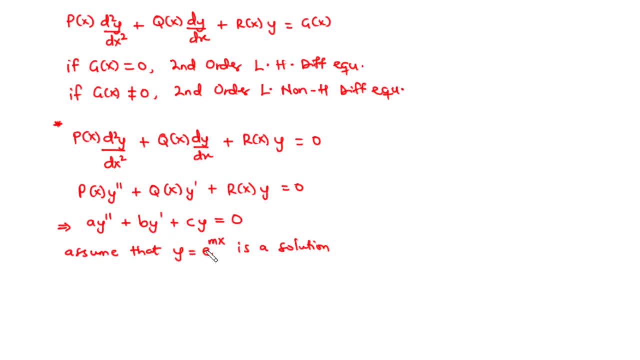 is that we are going to find y prime and then y prime prime from this function and then substitute that into the differential equation. So from this we can obtain y prime by differentiating this function. Now we differentiate the exponent with respect to x and then we have m. 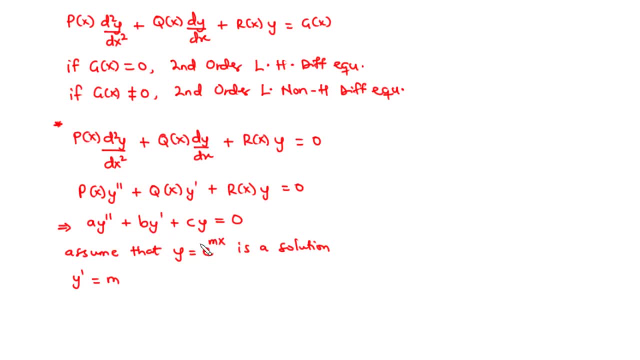 So the m appears here in front of the function, and then we are going to repeat whatever you have here, So that becomes times e to the power mx, And then if you want to find y, prime, prime, basically you are going to differentiate this. 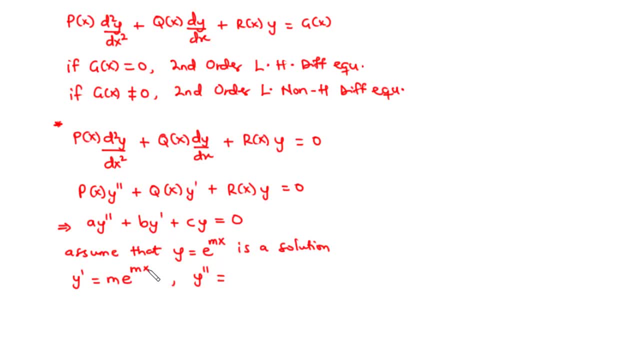 So you differentiate mx with respect to x, and then you realize that you have m. So you multiply m by m, and thus you have m squared times e to the power. you are going to repeat whatever you had. So e to the power, mx. 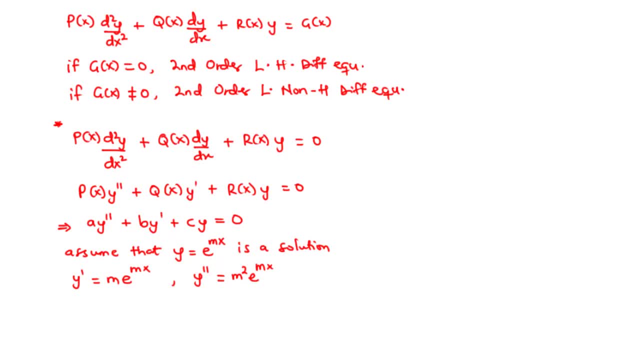 So this is y prime and this is y prime prime. The next thing we are going to do is to substitute these two into the original differential equation, So that you are going to have a times y prime prime, That is m squared times e to the power mx plus b times y prime, which is m times e to the power mx plus c times y, which is e to the power mx, equals 0.. 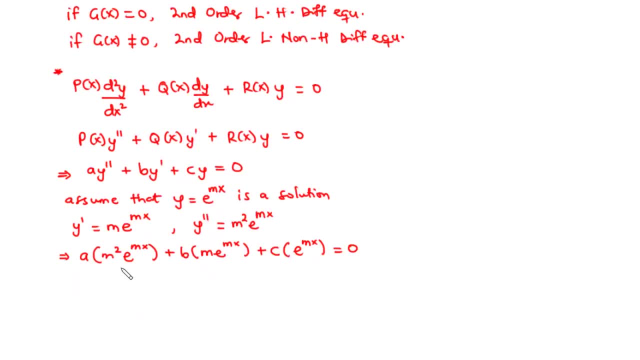 Now, at this point you realize that e to the power mx is common to each of the three things. So we can factor that out so that we have e to the power mx. on the outside, Inside of the bracket, we have m squared times, e to the power mx divided by e to the power mx. 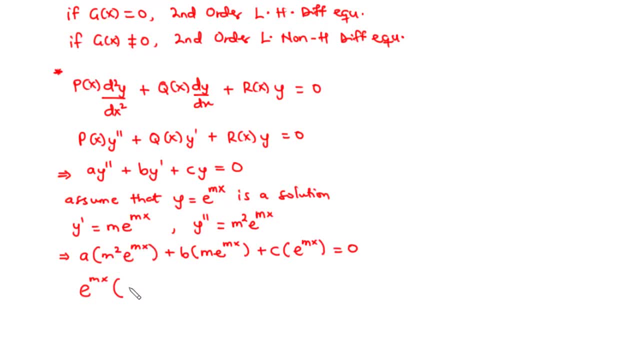 These cancels are this: We are left with am squared, So you have am squared plus. Now these cancels are this: We are left with bm Plus. these cancels are this: We are left with only c, And this is equal to 0.. 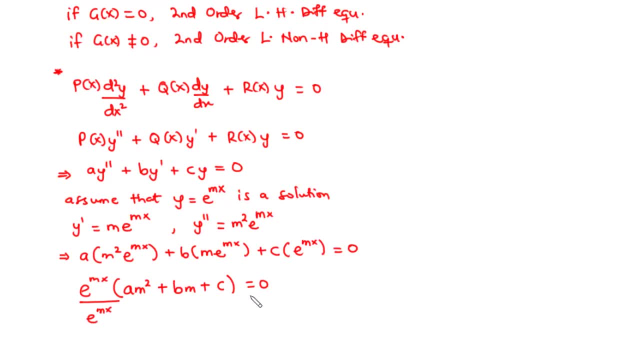 So we divide through by e to the power mx, e to the power mx, And then we are going to have am squared plus bm plus c equals 0. Now we call this the characteristic equation Or the auxiliary equation of the differential equation. 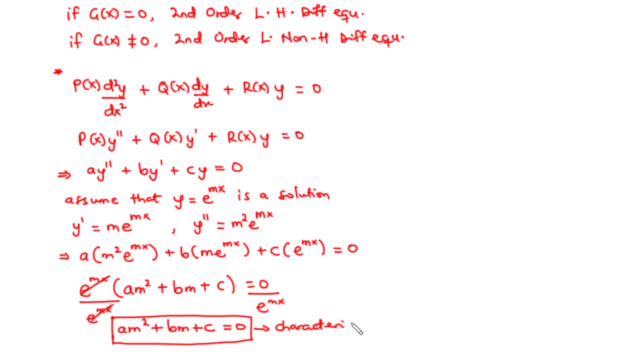 So this is the characteristic equation, Or, better still, the auxiliary equation of the differential equation. Now you realize that this is a quadratic equation, And hence the next thing we need to do is to obtain the roots of this quadratic equation. 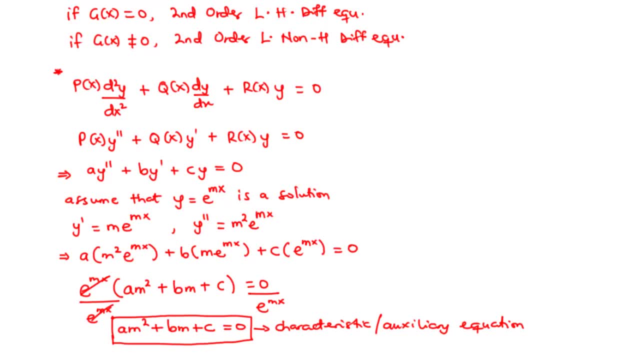 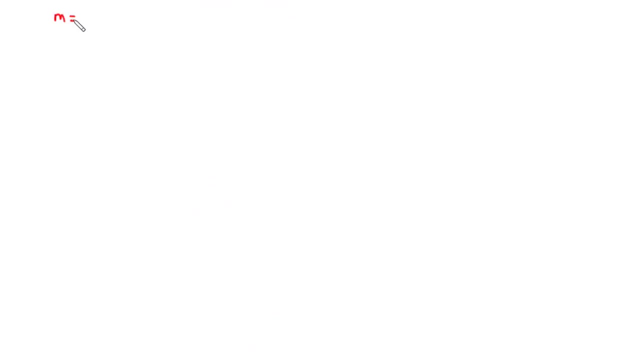 Or, better still, this auxiliary equation. Now, we can do this either considering the method of factorization Or, better still, using the quadratic formula. So, assuming you are using the quadratic formula, Then you can find the roots of the auxiliary equation to be equal to. 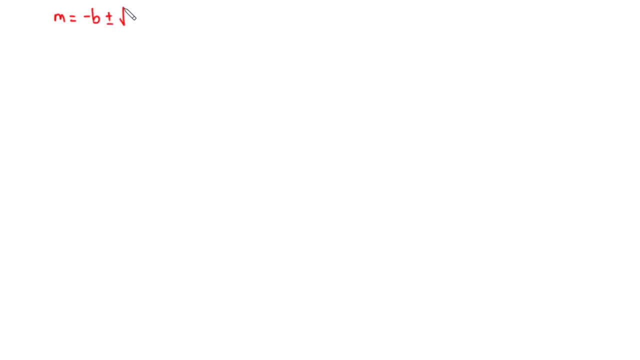 You have negative b, plus or minus the square root of b squared minus 4ac, all divided by 2a. So plus gives you one root and then minus also gives you the other root. Now, depending on the nature of the roots of the auxiliary equation, three possibilities may occur. 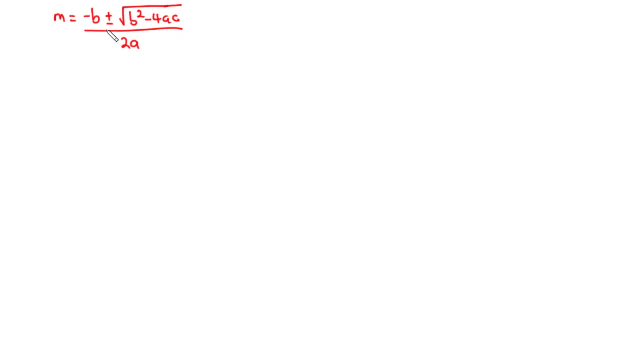 And we need to familiarize ourselves with these possibilities. So we are going to consider three cases here Which depend on the nature of the roots of the auxiliary equation. So if the roots, if the roots are, so we consider case 1. if the roots are real and unequal. 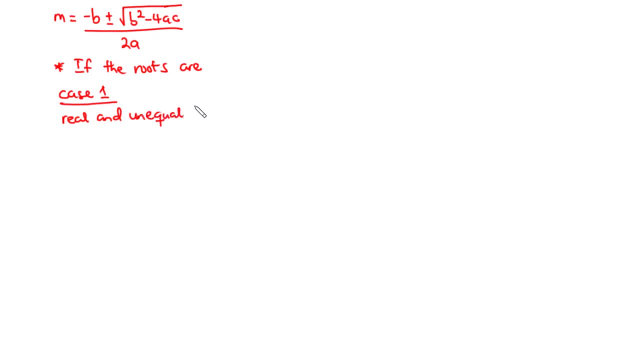 if they are real and unequal, or, better still, distinct, then we have m to be equal to m1 and we have m to be equal to m2, so that m1 is not equal to m2. now, if m1 is not equal to m2, then the 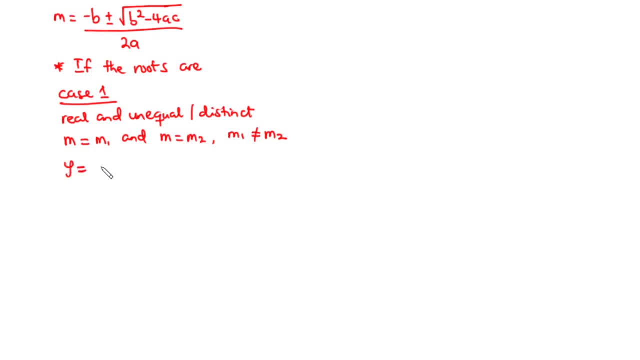 solution to the differential equation is given by: y equals c1 times e to the power m1 times x, plus c2 times e to the power m2 times x. now for case 2. case 2, that is, if the roots are real and equal. so this time, if the roots are real and 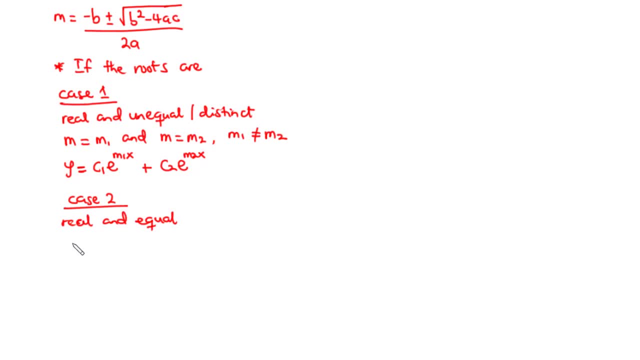 equal, then it means that m is equal to m1 and that is the same as m2. now, if we denote m1 with the double root, then we have the general solution, given as c1 times e to the power, m1 x plus c2 times x. 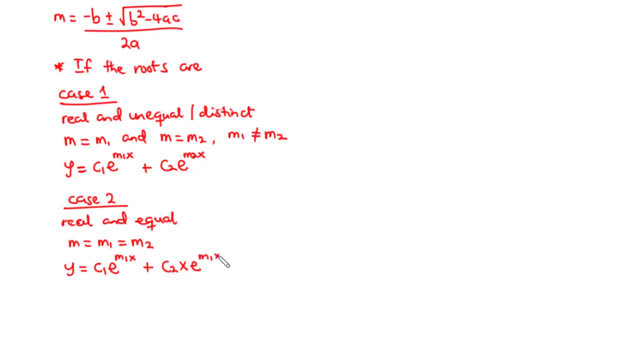 times e to the power, m1- x. again, if m2 is used to denote the double root, then instead of m1- m1 you are going to have m2- m2. now, literally, the value of m1 is equal to m2, so it doesn't really matter. 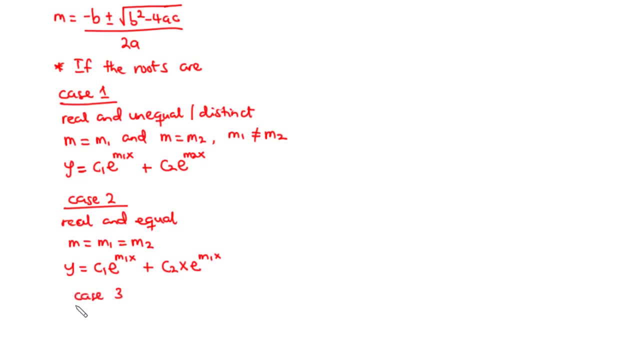 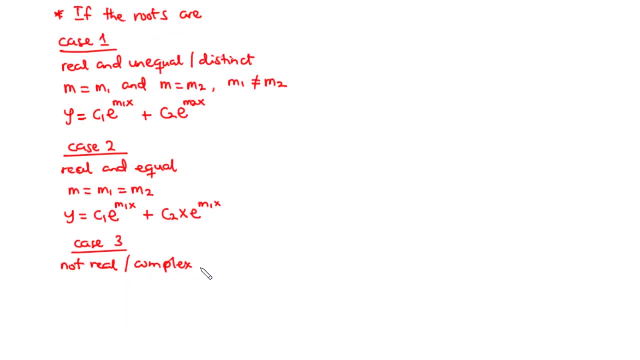 now let's move on to case 3. so for case 3, if the roots are not real, if this time the roots are not real or we say that they are complex, if the roots are complex, then that is where you have m to be equal to alpha plus or minus. i times beta. so with this you can have m1 to be equal. 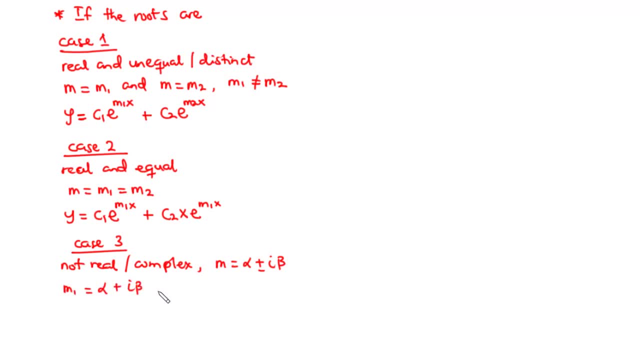 to alpha plus i beta and then m2 to be alpha minus i beta. now, with this the general solution is given by y equals e to the power alpha x times into brackets we have c1, cos, beta, x plus c2 sine. now the values of c1 and c2 for all three cases can be obtained. 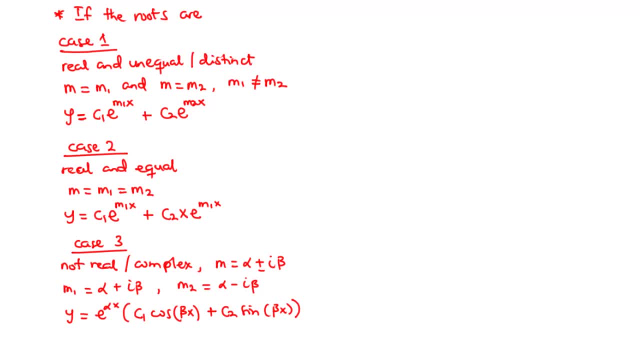 if we are given the initial conditions or, better still, the boundary conditions. now, in the next section, what we are going to do is to consider some examples covering all these three cases. so let's start by taking the examples, one after the other. so now let's start off with example 1. 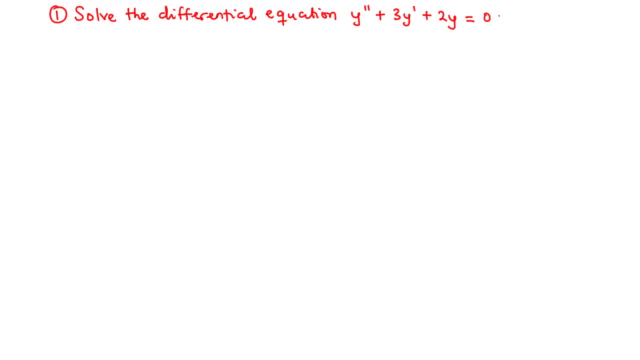 so in this example we are going to solve the differential equation y prime prime plus 3y prime plus 2y equals 0. so let's try to solve this together. so we have the differential equation y prime prime plus 3y prime plus 2y equals 0. 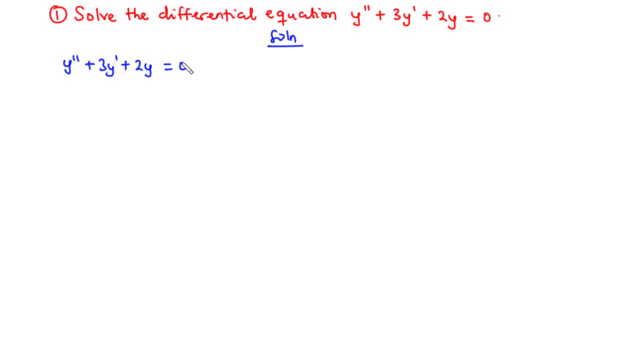 now to solve this differential equation, because we are dealing with second order linear, homogeneous differential equation where the coefficients are constant. we are going to solve this equation by doing the following: we can derive the auxiliary equation straight away from this differential equation. Now, to do so, we are going to replace y' with m2, y' with m and then y with 1.. 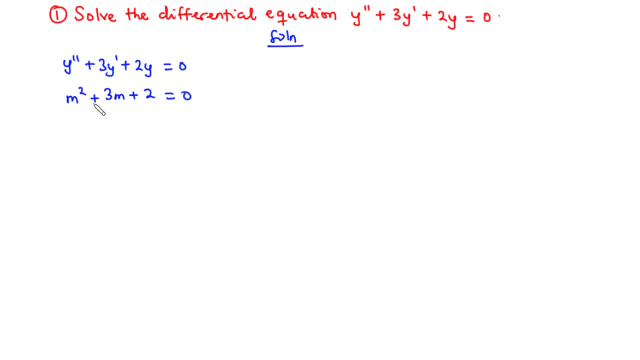 So you are going to have the auxiliary equation, or the characteristic equation to be: m2 plus 3m plus 2 equals 0. Now the next thing is to find the roots of this auxiliary equation. So we multiply the coefficient of m2, which is 1, by the coefficient of the constant, which. 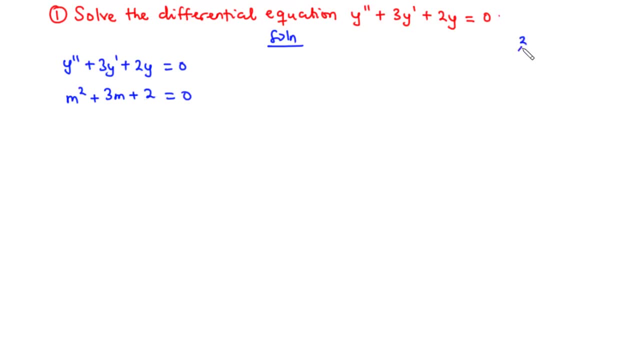 is 2.. So 1 times 2 is 2.. Now we need to obtain two numbers that when you multiply you get 2 and then when you add you get 3.. That is simply 1 and 2.. So 1 times 2 is 2, 1 plus 2 is 3.. 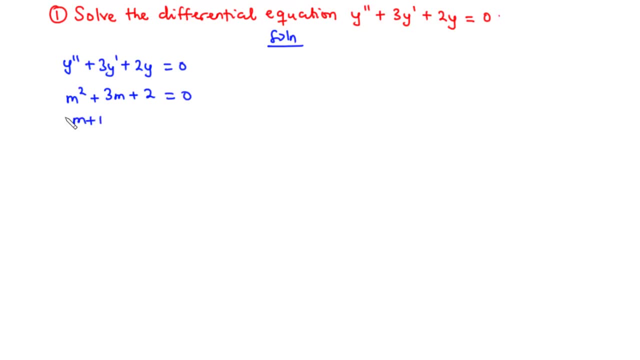 So we have the factors to be m plus 1.. And then we have m plus 2. So that is equal to 0. So first we have m plus 1 equals 0. We have m equals negative 1.. And then next, we have m plus 2 equals 0, and then we have m equals negative 2.. 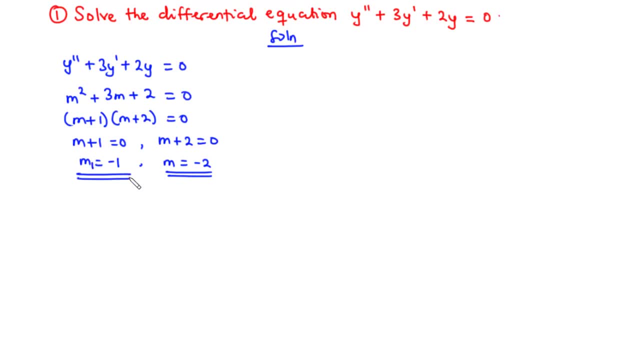 So we can call this m1.. And then we call this m2.. Now, since the roots are real and unequal, Let's think about this equal. then we say that the general solution is given by: y equals c1 times e to the power. 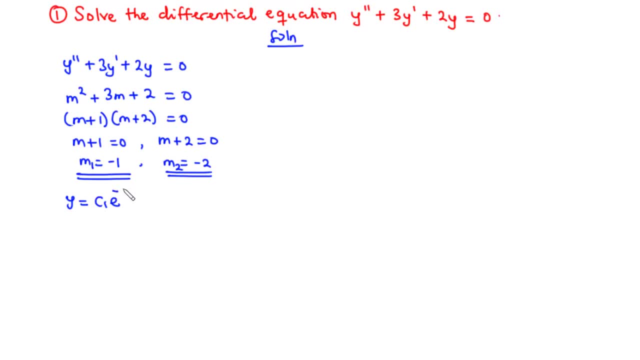 m1x, So we have negative 1 times x, which is negative x plus c2 e to the power m2x, So that is negative 2x. So this happens to be the general solution to this differential equation. So now let's move on to the next example, That is, example 2.. In this example we are asked to solve the 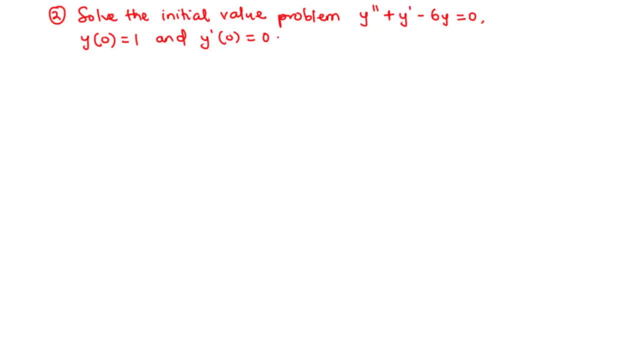 initial value problem: y prime prime plus, y prime minus 6y equals 0.. We have y of 0 equals 1 and y prime of 0 equals 0. So let's solve this. So we have the differential equation y prime prime. 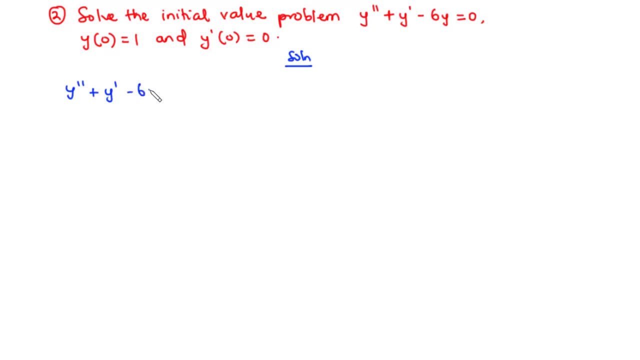 plus y prime minus 6y equals 0. Here also we can obtain or derive the auxiliary equation straight away. So here this becomes: m2 plus m minus 6 equals 0. So we multiply the coefficients of m2, which is 1, by negative 6, and then we have: 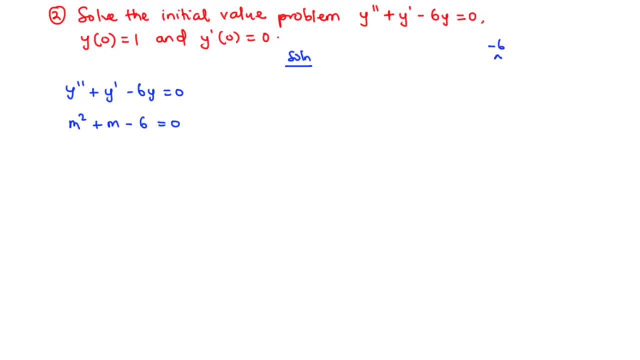 negative 6.. We want to find two numbers that when you multiply you have negative 6 and then when you add you have 1.. So first we have, let's say we have- 1, 6, we have, let's say, 2 and then 3. So we can make this negative 2 and then plus 3.. So when you 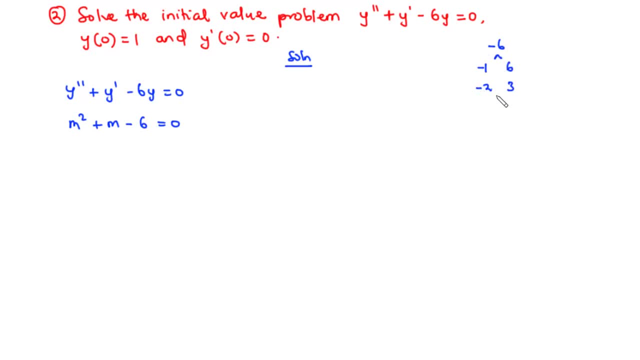 multiply these two numbers, you have negative 6. When you add them you have 1.. So we are going to use negative 2 and then 3. So we have the factors to be: m minus 2, m plus 3 equals 0. So first we 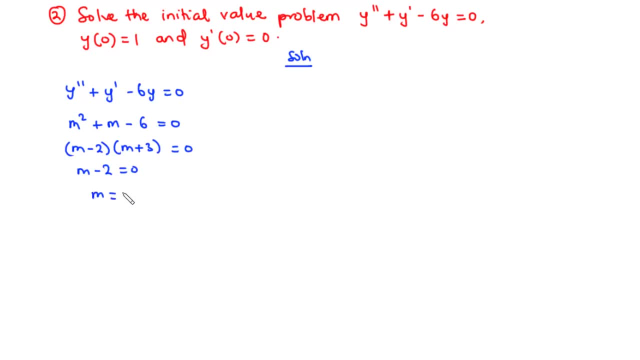 have: m minus 2 equals 0.. m is equal to 2.. And then m plus 3 equals 0.. m is equal to negative 3.. So let this be m2.. We have this to be m1.. Therefore, since the roots are unequal, they are real and unequal. then you have y to be equal to c1, e to the power 2x. 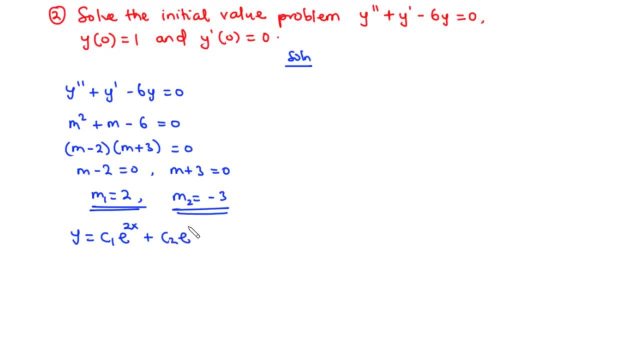 plus c2 e to the power negative 3x. So this is the general solution of the differential equation. Now we are given the initial value conditions and we need to solve further to obtain the particular solution of this differential equation. So what we are going to do is: 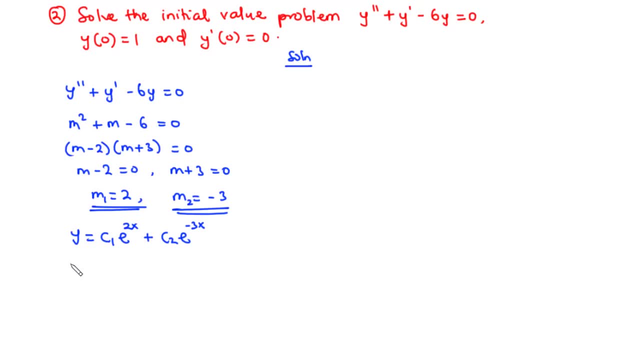 here we have y of 0 equals 1.. So we say for y of 0 equals 1, what this parameter means is that we have the value of x to be 0. And then we have the value of y to be 1.. 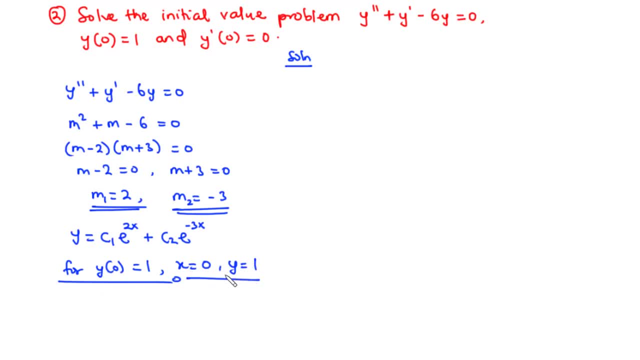 So we are going to plug x equals 0, y equals one into the general solution, because this is y and then we have values of xa. So that becomes we have 1 equals c1 times e to the power, 2 times 0, plus c to e to the power, negative 2x. and so on until you have x to be zero equal to 1.. Now we stupidly stay here and we have to remove 2x from the equation. We put y to be 0 equal to xa and dW per 1 x, e to the power 2x. If we subtract these two numbers it will take us 300 times the value of x. So we plug x to the power equal 2x plus c2, e to the power negative 4x, And then we Inform the vão of the derivative equation, which is x and 2's. 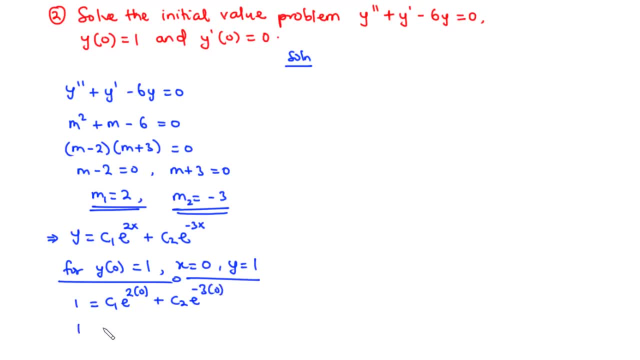 power negative three times zero. so this becomes one equals. now, two times zero is zero. and then e to the power zero is one. any non-zero number raised to the power zero is equal to one. so we have one times c one which is c one. the same happens to this term, so we are going to have plus. 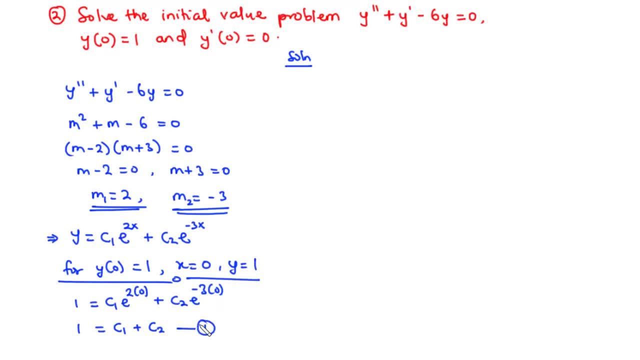 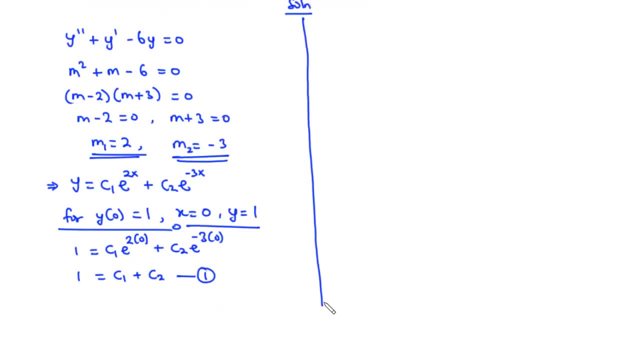 c two. so you call this equation one. so the next thing is: the next thing is for y prime of zero, equal zero. we have X to be equal to zero. we have Y prime also to be equal to zero. so you are going to plug in: first of all we are going to find Y prime, and then you're going to find my third. 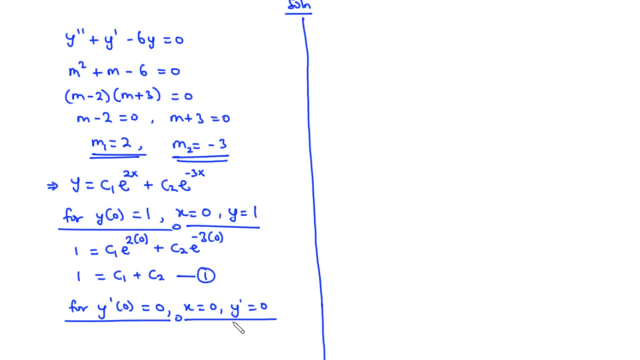 then we plug in: x equals 0 and then y prime also equals 0. So we are trying to find the first derivative of this general solution, so that becomes y prime equals. we are going to differentiate this with respect to x, so we have 2, so it becomes 2c1 times e to the power 2x, and then this becomes. 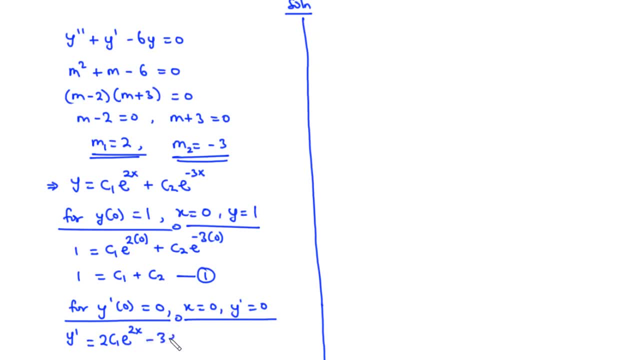 negative 3 times c2. e to the power, negative 3x. so we have y prime equals 0. so on the left hand side we have 0 equals now 2 times 0 is 0. e to the power, 0 is 1, so that becomes 2 times c1 minus. 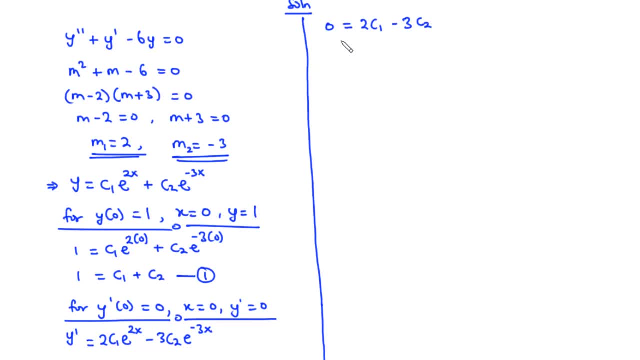 3 times c2. so you can transpose negative 3 c2 to the left hand side so that we have 3 c2 equals 2 c1. we divide 3 by 3 by 3 and then we have we have c2 to be equal to 2 over 3 times c1. 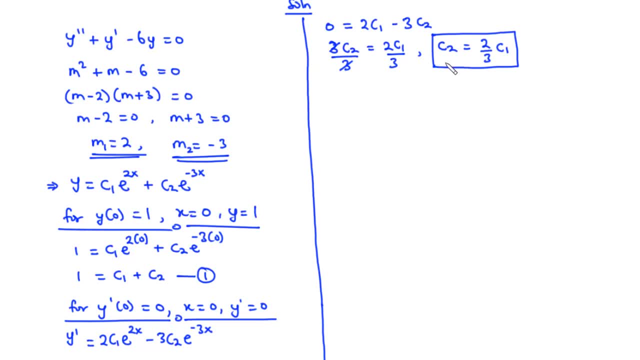 so the next thing is we are going to plug in c2 into equation 1, so we put c2 in equation 1. so for equation 1 we are going to have 1 equals c1 plus c2. we have 2 over 3 c1. 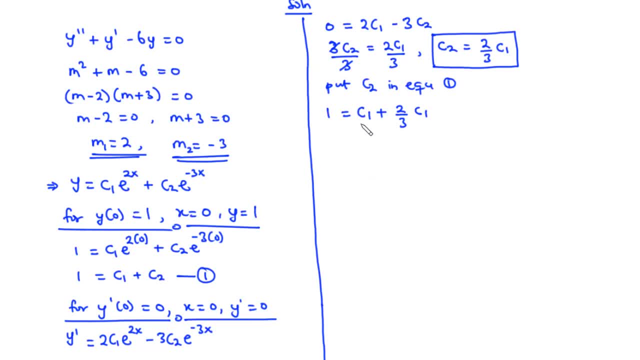 so you want to find the lcm. you want to find the lcm. so lcm between 1 and 3 is 3. 3 divided by 1 is 3. 3 times c1 is 3. c1 plus 3 divided by 3 is 1. 1 times 2 is 2. so we have 2 c1 and that is equal to 1. so we cross multiply. 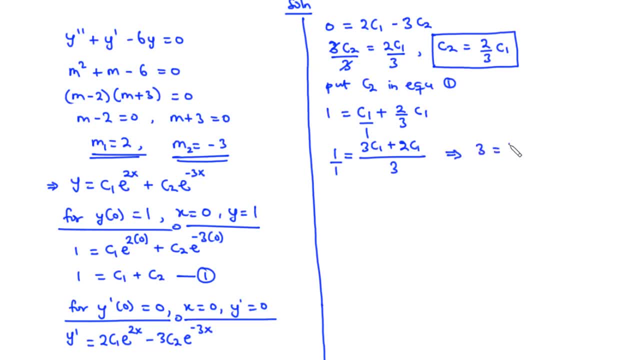 and then we have 3 on the left hand side equals 3 c1 plus 2 c1 and that is equal to 5 c1. we divide 3 by 5 by 5 and you realize that we have c1 to be equal to. 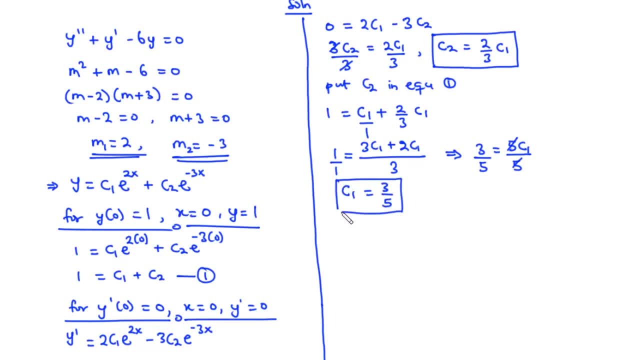 3 over 5. so this is the value of c1. and then for c2, c2 is equal to 2 over 3, c1, so 2 over 3 times 3 over 5. these cancels are this: we are left with c2 to be equal to 2 over 5. 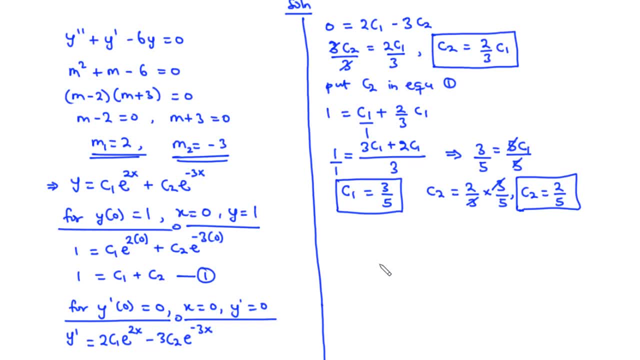 so this is the value of c2. now we can write the particular solution, that is, from this we have y equals c1, which is 3 over 5 times e to the power 2x, plus c2, which is 2 over 5 times e to the power negative 3x. so this happens to be the particular solution. 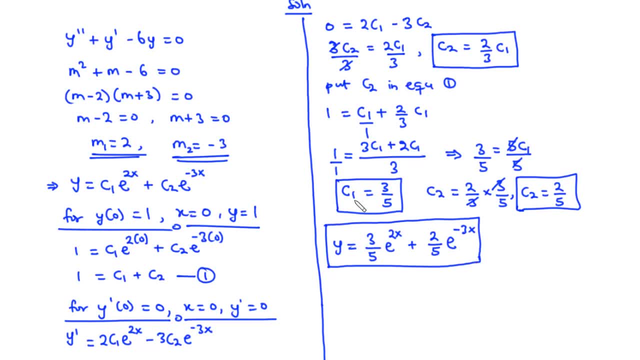 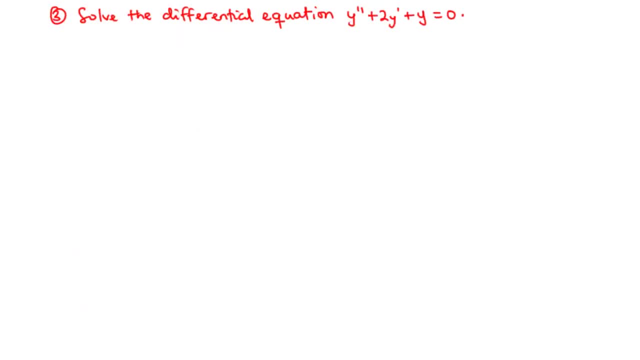 of this differential equation, given the initial conditions. now let's move on to the third example. so in the third example we are going to solve the differential equation y prime prime plus 2y. prime plus y equals zero. so we have y prime prime plus 2y. prime plus y equals 0, so this becomes m square plus 2m plus 1. 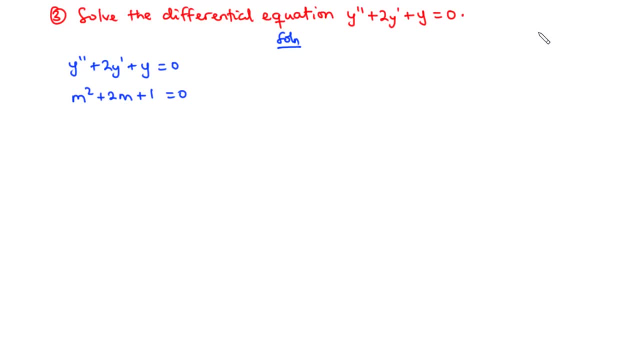 equals 0.. we multiply 1 by 1, so that is 1. we want to find two numbers that when you multiply you have one, when you add you have two, so that is basically one, and then one factors to be m plus 1. m plus 1, that is equal to 0, so this becomes m plus 1. 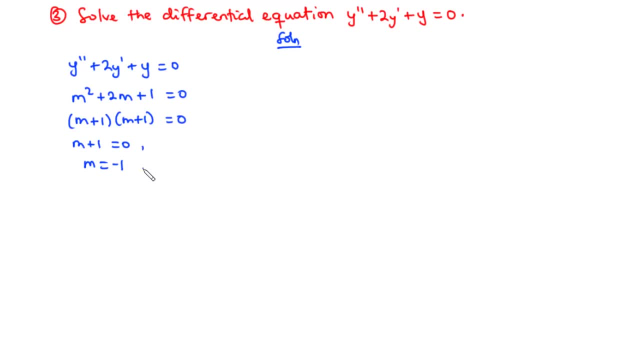 equals 0, m is equal to negative 1, and then m plus 1 is equal to 0. we have m equals negative 1. so here we have m 1, we have this to be m 1, we have this to be m 2, and you realize that m 1 is equal to m 2 and that is equal to negative 1. so 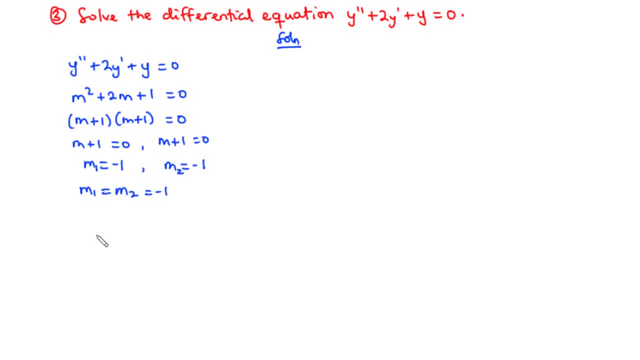 here you realize that the roots are real and they are equal. they are equal roots, real and equal roots. so the general solution is given by: y equals C, 1 times e to the power negative X, plus C 2 times X times e to the power negative X. this: 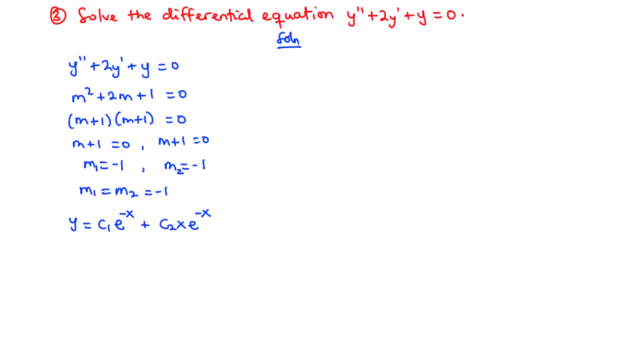 is the general solution to this differential equation. now let's move on to the last example, where we are going to solve the differential equation. y prime prime minus 6y prime plus 10y equals 0. let's solve this together as well. so you have y prime prime minus 6y. 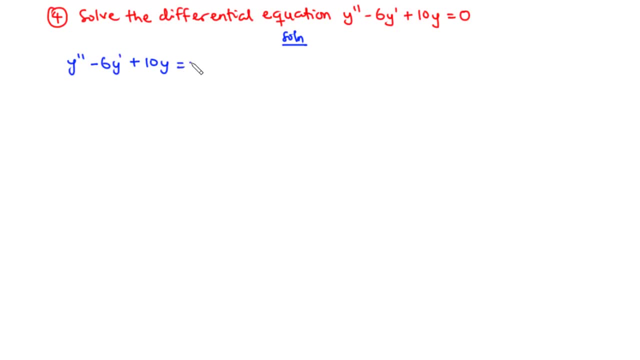 prime plus 10y equals 0. so this becomes m square minus 6m minus 6y plus 10y equals 0, so this becomes m square minus 6m minus 6m plus 10, and this is equal to 0. you multiply the coefficient of m square by: 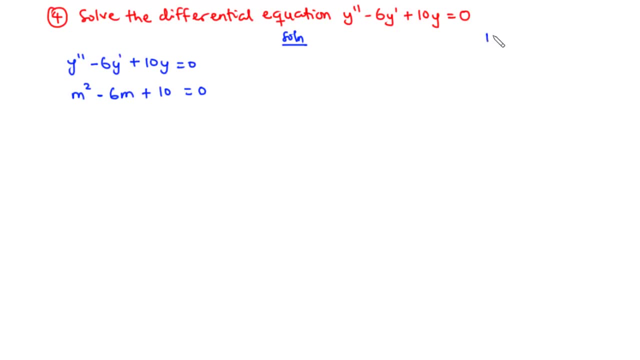 the coefficient of the constant. so 1 times 10 is 10, and then you want to find two numbers that when you multiply you are going to obtain 10, and then when you add you have negative 6. so let's say we have factors of 10, we have 1, then we 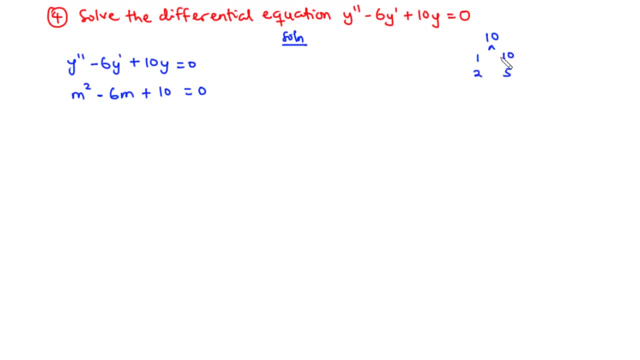 have 2, 5 now, out of these two sets of numbers there is no way you can add any degrees here. so you only have 1. every point, you have a zero, so you spare one point, and that's what M can do, that's adding free respect. and then you have 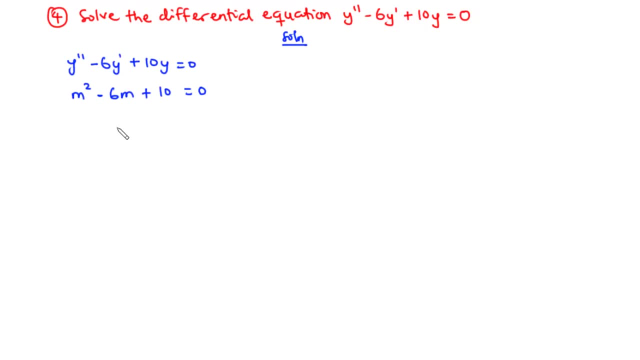 m squared because it's in terms of now our the e to the power negative x, 삼 square in właści petite alpha: 1 to e to 2, 것이 g, b for y to the power negative six. so you can see we are going to use m flat. which is given by b, u to be equal to negative b plus or minus the square root of for and divided by 2a. now we have a to be one coefficient of m squared 1. price per m square is 0 to chl square for a, pero, a, c, all divided by 2a. now we have a to be one coefficient of M squared 1, andитуated everything to cover all of these y, the exact point we're going to use. same case: 1, n equals to be n plus some at our e to the Yang coefficient. tally the channel machine: An's equation. now Description: 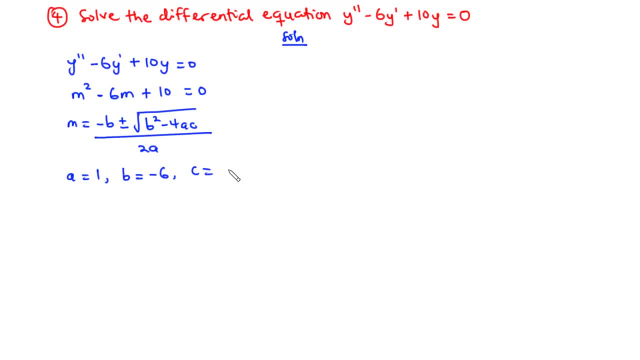 we have b to be negative 6. we have c to be 10. so let's plug in the values a, b, c. so we have m to be equal to negative negative 6 plus or minus. we have the square root of negative 6 square minus 4. we have a to be 1. we have c to be 10, or divided by 2a. 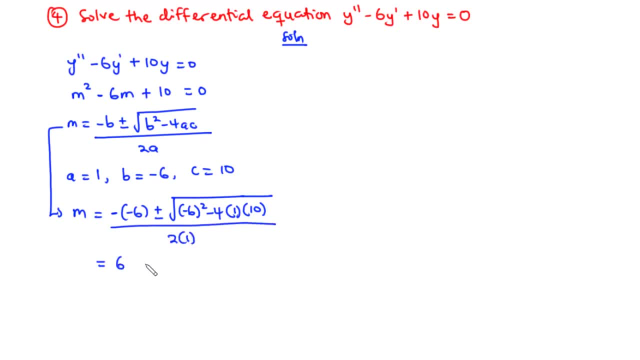 so this becomes 6 plus or minus square root of negative 6. square is 36 negative 4 times 1. negative 4 times 10 negative 40 or divided by 2, so this becomes 6 plus or minus square root of negative 4, or divided by 2. 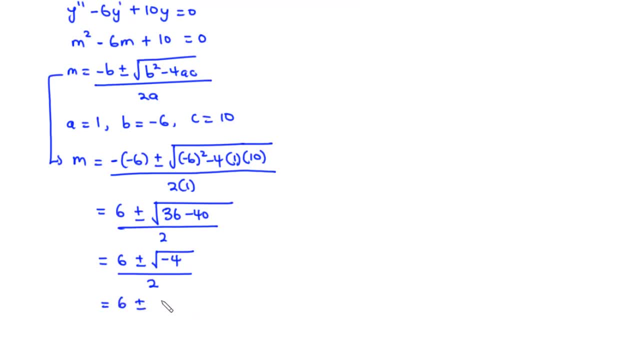 and then we can express this as square root of negative 1 times square root of 4 or divided by 2. so here we can express this as six plus or minus. square root of negative 1 is i, the complex number or the imaginary value i, and then square root of 4 is 2.. 4 divided by 2.. So we can simply express this as 6 divided. 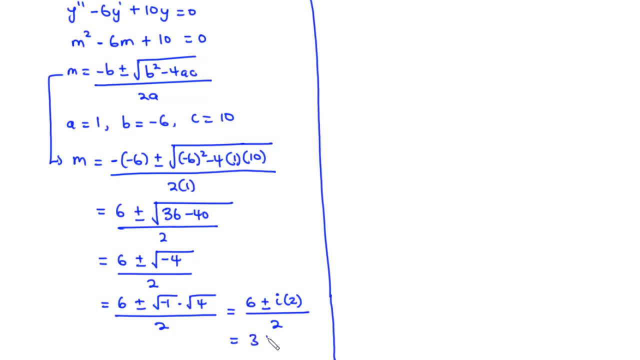 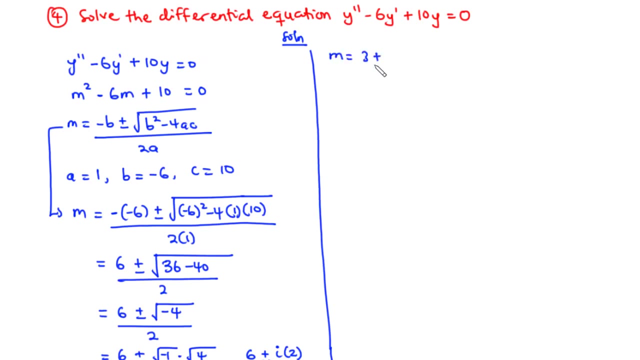 by 2 is 3.. So 3 plus or minus 2 divided by 2 is 1.. So 3 plus or minus i. This is the value of m. This is the value of m. So we have m to be equal to 3 plus or minus i, which is equal to alpha plus. 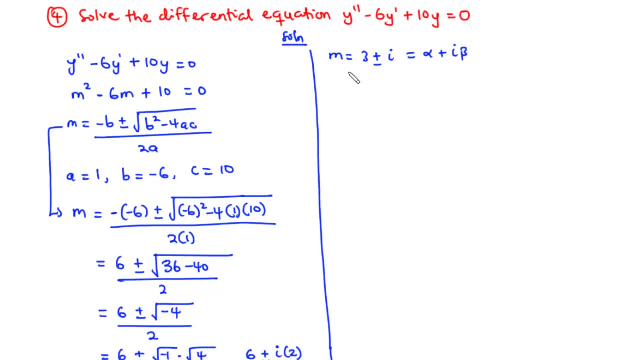 i beta. So what this primarily means is that we have alpha. This is plus or minus, So we have alpha to be 3 and then we have beta to be 1.. Now, since we have a complex root, then the general solution is given by y equals e to the power, alpha x into brackets c1.